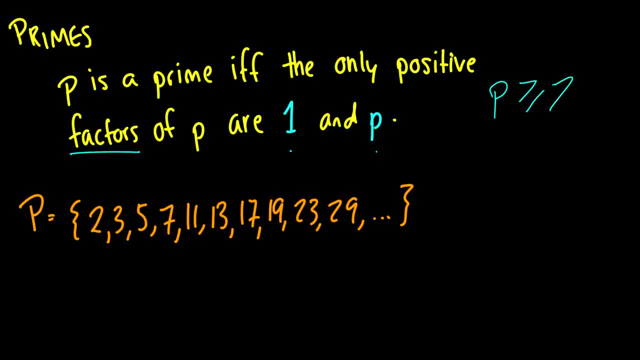 So it's sort of simple. Of course, primes are only greater or equal to 2.. 1 is not a prime number in this case, So we have a nice set here: 2,, 3,, 5,, 7,, 11,, 13,, 17,, 19,, 20,, 23,, 29.. 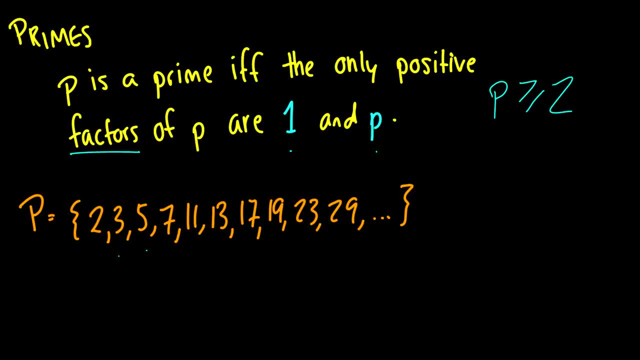 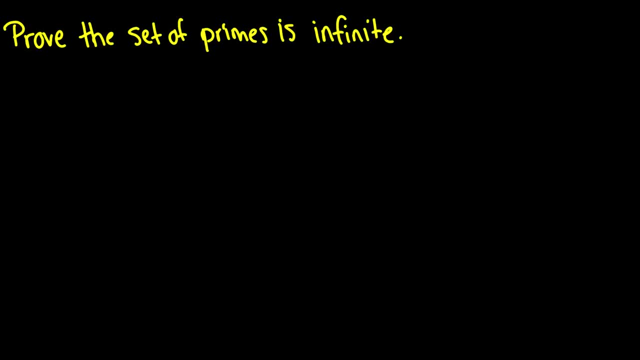 They go on and on, For instance, 31,, 37,, 41. You can go on a long time with prime numbers. So I'll do a pretty well-known proof. In fact, I'm surprised if you haven't seen this already. 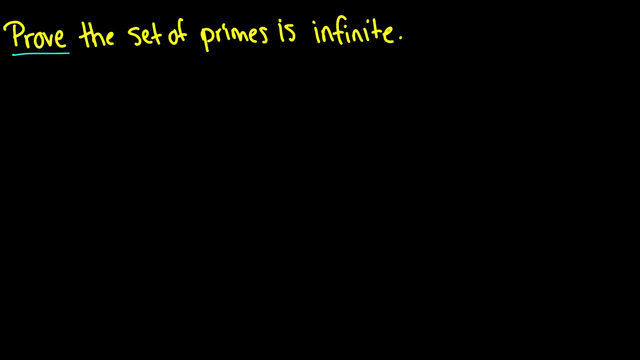 And we prove that the set of primes is infinite. So what we'll do is we're going to assume that, well, the set P is finite, And of course we say the set P. In fact, we'll write this, We'll write P1, all the way. 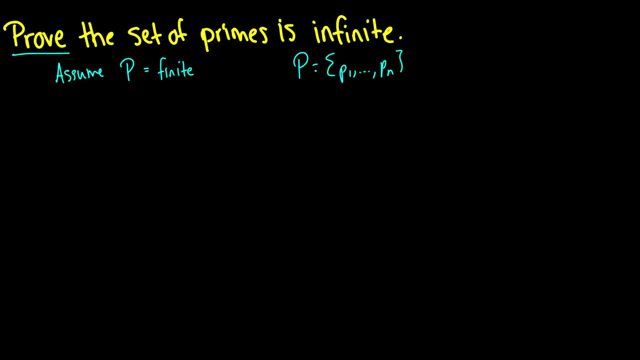 All the way up to Pn, And these P's are going to be prime numbers. So clearly, P1 is going to be 2. And Pn- we don't know which one it is because we don't know what the highest number is. 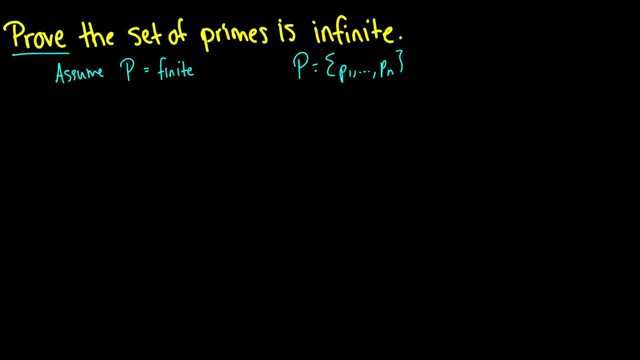 But we're saying that there is a last prime number. Okay, So what we'll do now is we'll say: let's define a new number. Let's take Pn plus 1. And this is going to be P1.. P1 times P2, all the way up to Pn. 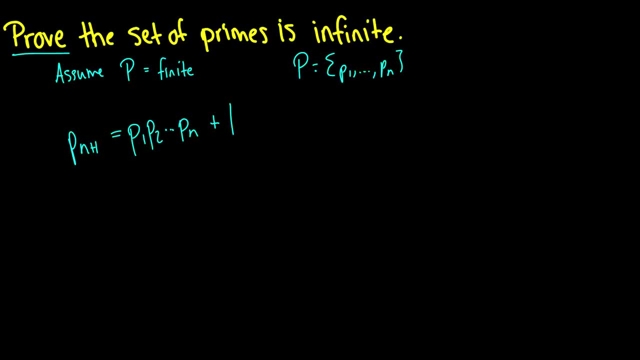 And then we're going to add 1.. So what we know about division is that this implies that Pn plus 1 is prime, Because these other prime numbers are all of its factors. But then if you add 1, well, P1 plus 1 can't divide. 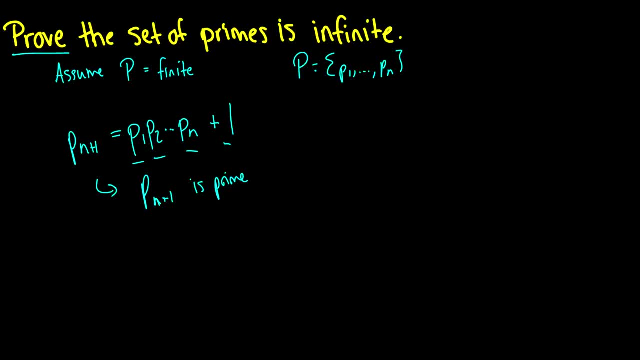 Well, like you can take any subset and you can add 1. And then it can't really divide this number, Pn plus 1.. So that means that Pn plus 1 is prime, But the problem is that we assumed it was finite. 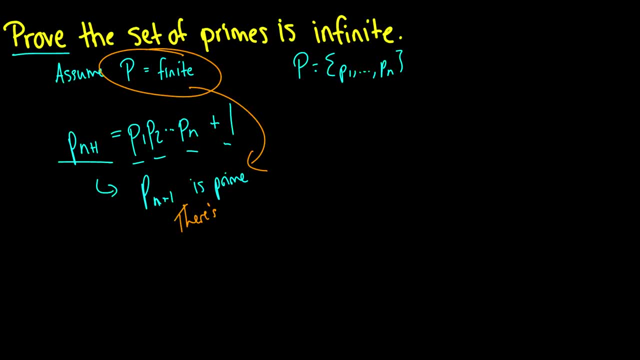 But what we're saying is that, no, there's one more. So, by contradiction, we know that, therefore, it's infinite, And this is a very famous proof. In fact, it's probably If you were introduced to, If you were introduced to one of the proofs at the beginning of your course. 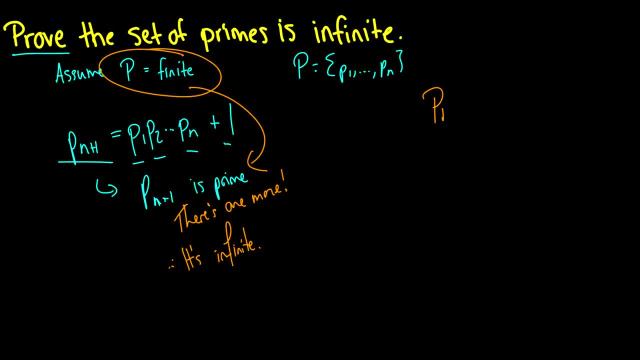 and say, hey, this is what we're going to do in this course. you either do this prime proof or you do the root 2 irrational proof, Because these are the nicest proofs that you can teach, that are very easy to understand and are actually pretty cool proofs. 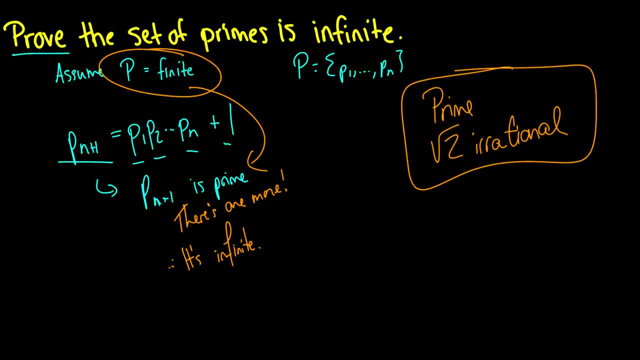 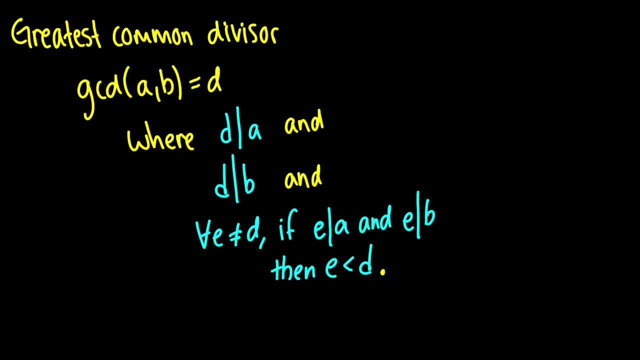 So you've probably seen this before. If this is your first time, this is probably something you would not prove in an exam, because you're taught it pretty blatantly Almost in any class you take. So let's talk about greatest common divisors now. 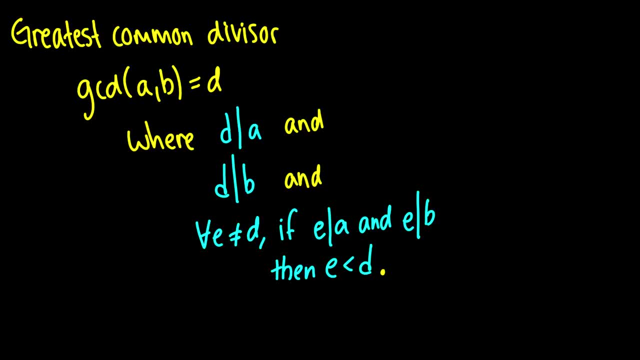 Now that primes are over. So we say that the greatest common divisor of A and B is equal to D, And this means that D divides A, D divides B And for any other divisors of A and B, if E divides A and E divides B. 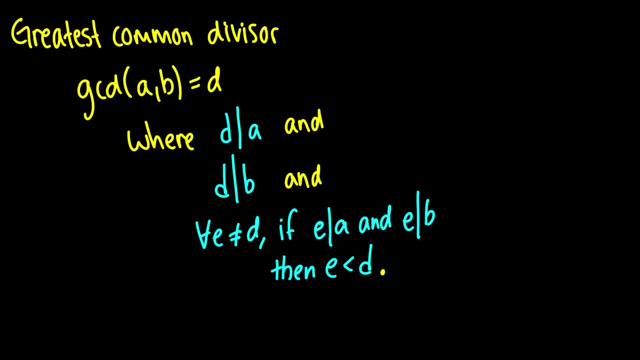 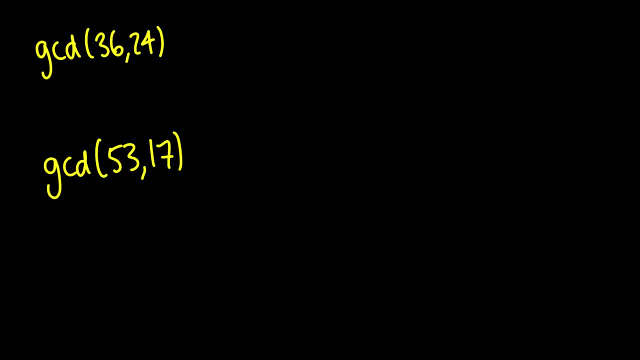 then E is going to be less than D. So of course, this is kind of a really garbled amount of information and saying: well, what does this mean? Let's take the numbers 36 and 24.. What we're saying is: we want to find the largest number. 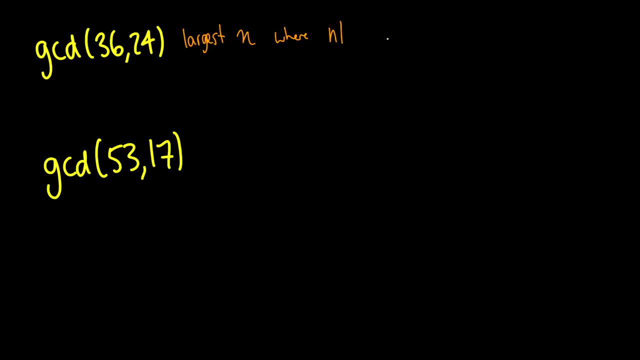 so the largest N, where N divides 36 and N divides 24.. That's what we want to find And it has to be the largest. So we can start out. Let's say we want to put 2.. So we know 2 divides 36 and 2 divides 24.. 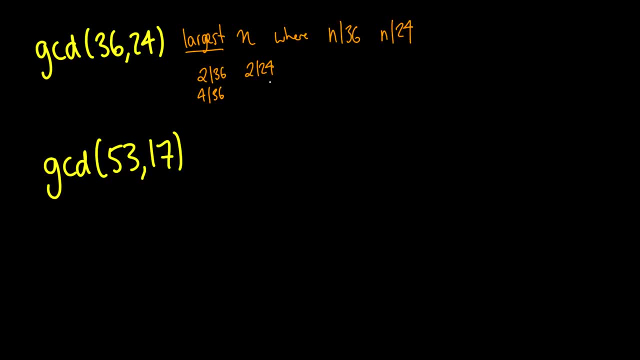 But I think we can do better. In fact, I think we can see that, OK, 4 divides 36 and 4 divides 24 as well, And we can keep going until we find that, hey, well, actually 12 divides 36 and 12 divides 24.. 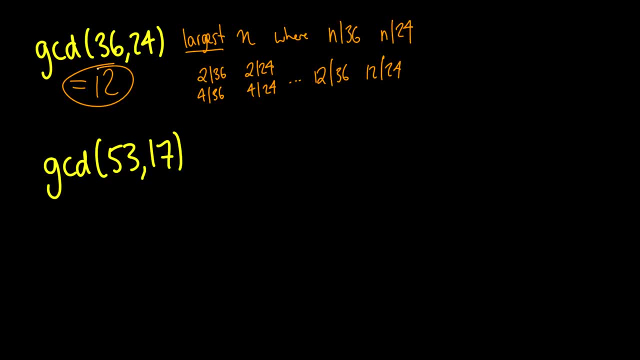 And there's no number greater than 12.. Therefore, this number is equal to 12.. Now here's another good question. Is that: how do you find these numbers? And don't worry, we'll figure out a way to figure that one out. 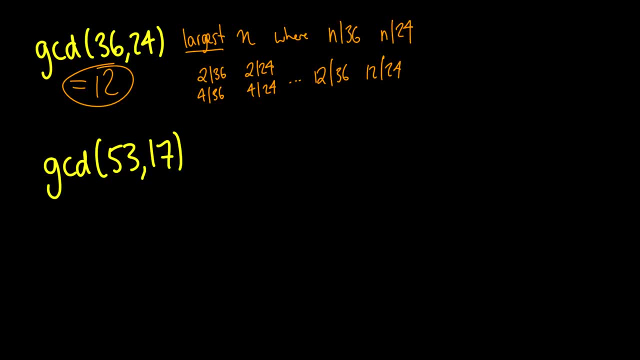 in a video or two from now, But for now we're using simple numbers just to get the idea of what it means. So here's a question: What is the greatest common divisor of 53 and 17?? Well, the first thing you probably want to check: 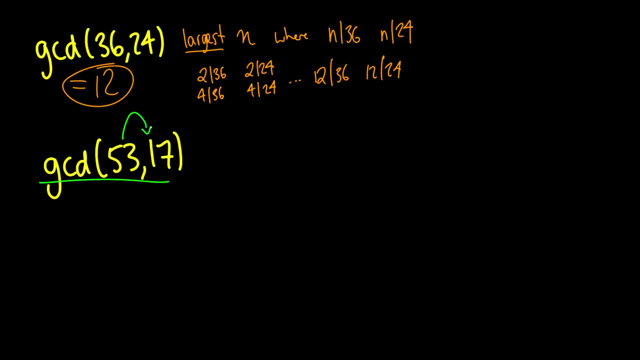 in fact this is a very good idea- Is to try to divide one number by the other and see if it fits. Because if I had, say, the GCD of 50 and 10, well, 10 divides 50.. 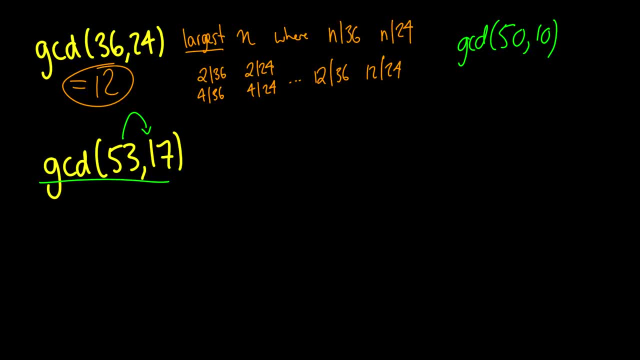 So clearly it's going to equal 10.. But in this case we see that no, it's not the case, that 17 divides 53. So I'll keep moving on. And then we say, OK, well, what are the factors of 17?? 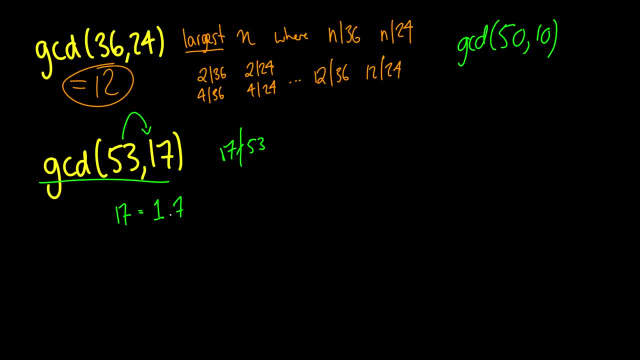 And it's interesting because the only factors of 17 are 1 and 17.. So if 17 doesn't divide 53, then the only number that can divide them both is going to be 1.. So the GCD of 53 and 17 is just going to equal 1.. 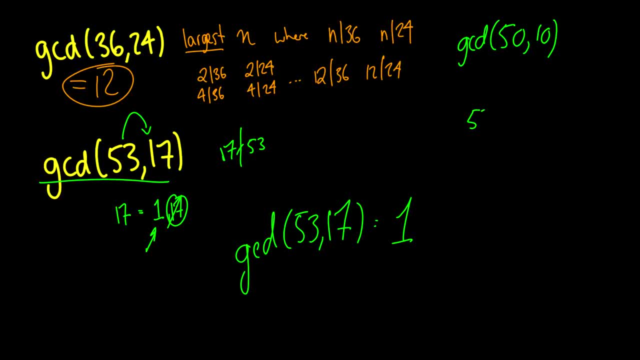 And, of course, if you checked out 53,, you'd also see that it's prime. So if you list out the common factors of them both, you'd see that it's prime. So you'll get 1,, 53,, 1, and 17.. 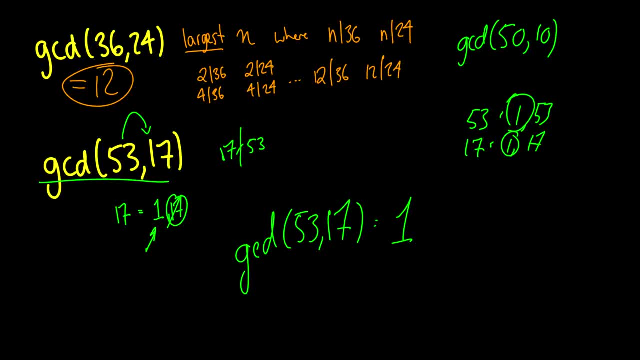 You find the highest common pair and you call it a day. In fact, we could have done that for 36 and 24.. You just list out all the factors and then you circle the highest common one, which is something you do in high school. 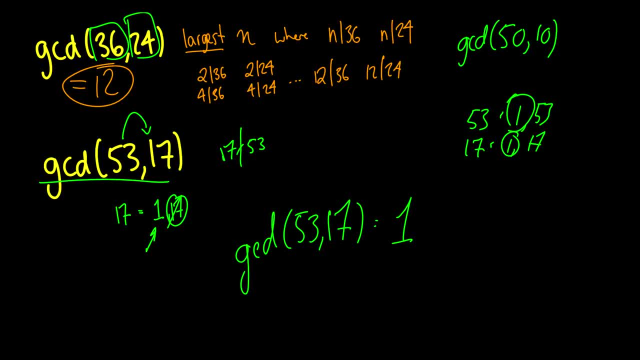 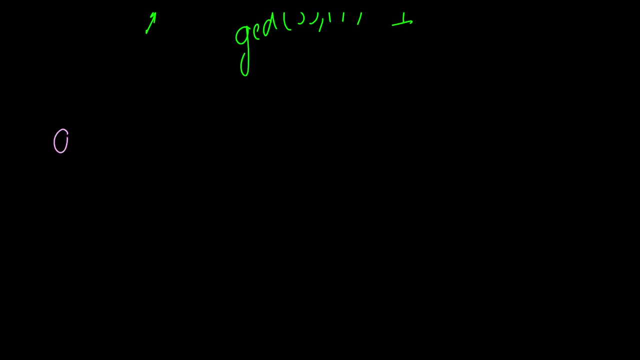 or elementary school or whenever you learned it. So that's a nice way. except imagine now that we have a little bit of a crazier number And I say, OK, find the greatest common. It's a denominator of 17,184 and 31,618..